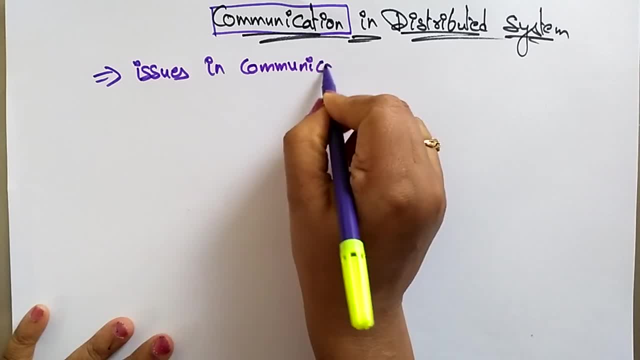 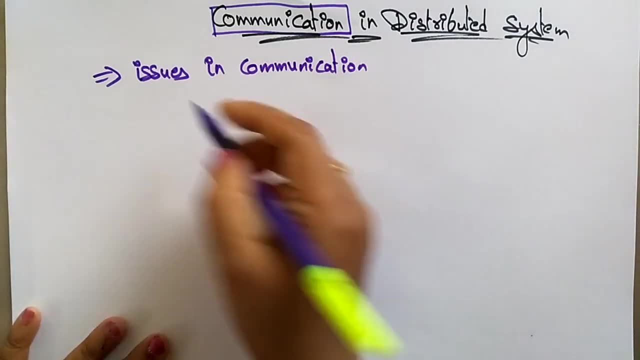 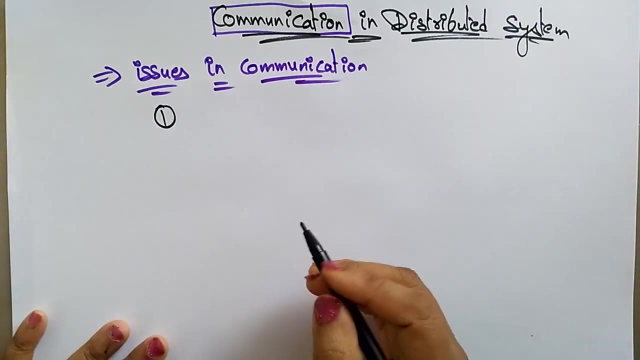 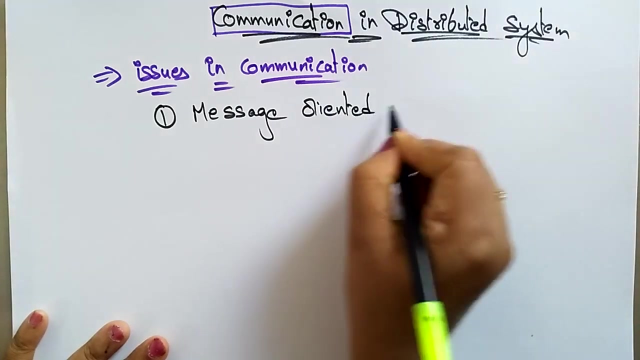 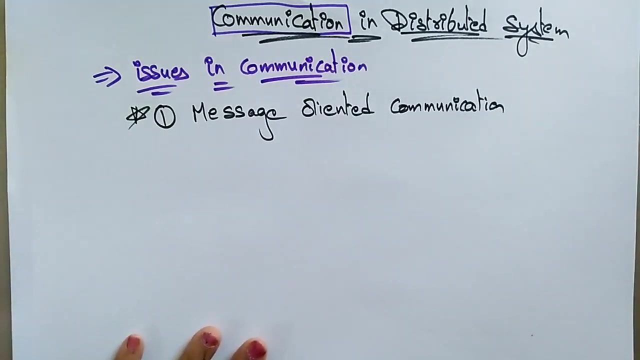 communication, then you can easily understand how you can establish a communication in distributed system. So what are the issues in communication? The different issues in communication is: first, is message oriented communication, Message oriented communication. So this is one of the most important issue, while when we are discussing about the communication, Message oriented communication. 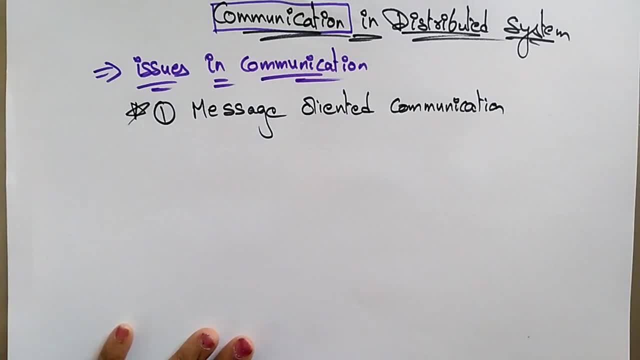 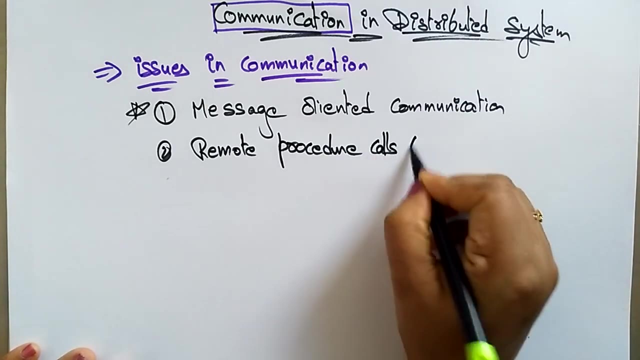 How the message is going to be communicated from one end to the another end. So this is one of the issues. And next, remote procedure calls. Remote procedure calls, So we call it as RPC. So the remote procedure call is another issue in communication. So when we are talking about the communication, we need to 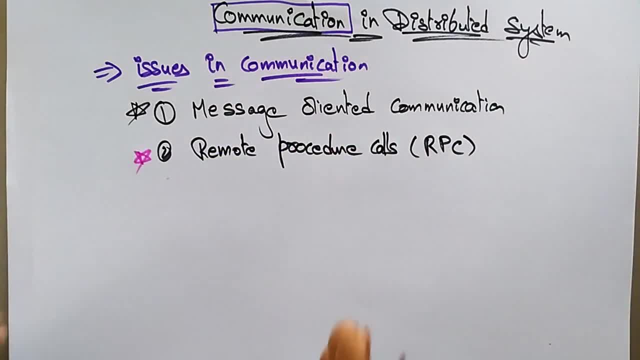 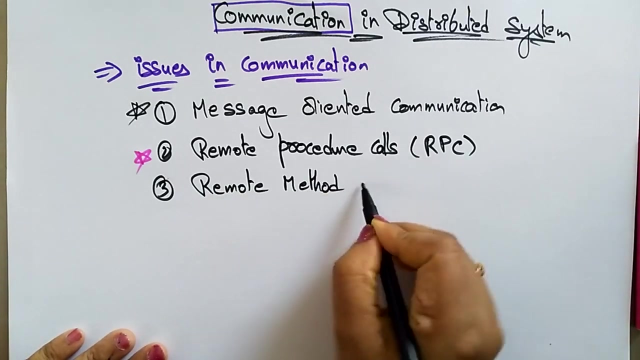 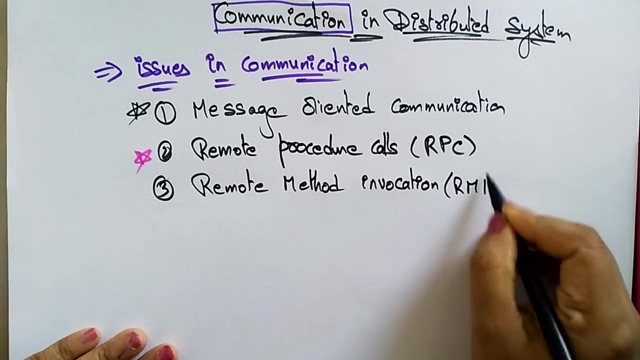 know what is this remote procedure call. So the remote procedure call here: the transparent. it maintains transparency, but poor for passing the references. Okay, And another thing. Another issue in communication is remote method invocation. Remote method invocation, like in our language, can be a problem. So what? these communication? Mouse catch, Horse catch Or om salt seis on 45s I just then Invocation. so this is a type of communication. so this is one of the issue that the communication has to be established in the data distributed system. So this is all the different types of communication in distributed system: message oriented, RPC, RMI. So RMI are essential. let me write that, or well as I. 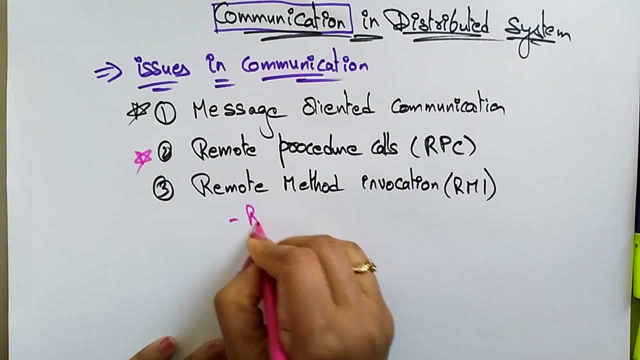 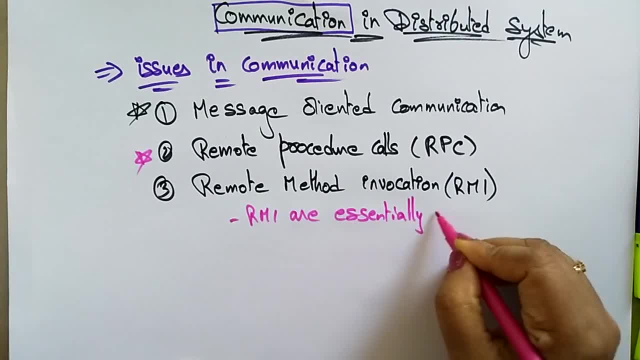 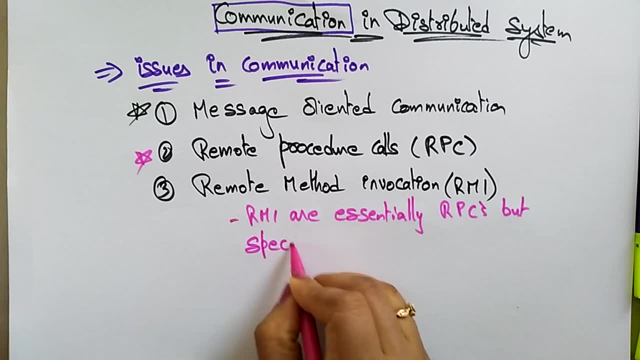 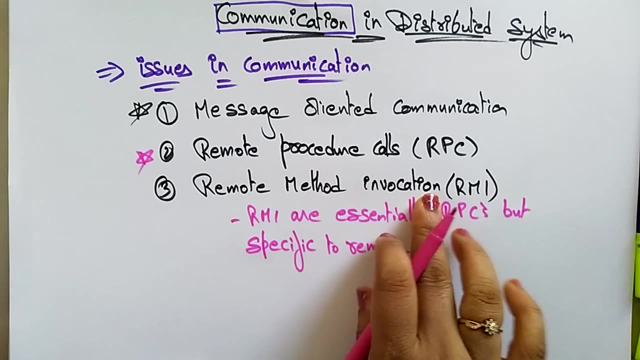 Are- and I and I essential- essentially RPCs, but specific to the remote object, but specific to remote objects. So RMI, that is, the remote method invocation, is mainly specific with the remote objects. Here the system wide reference passed as a parameters. 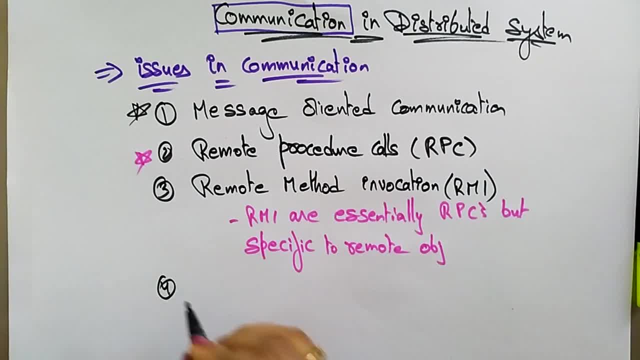 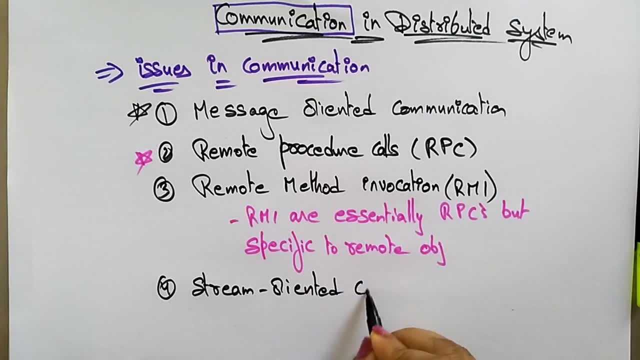 And another type of communication that is stream oriented communication. So these are all the different types of communications that in distribution, that are there in distributed systems, So message oriented communication, remote processor calls, remote method, invocation and stream oriented communication. So we will discuss one by one, clearly with an examples. 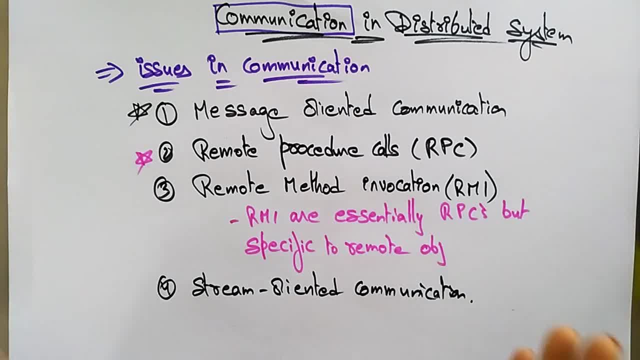 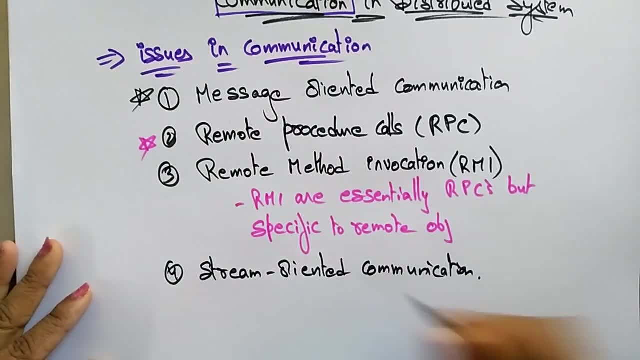 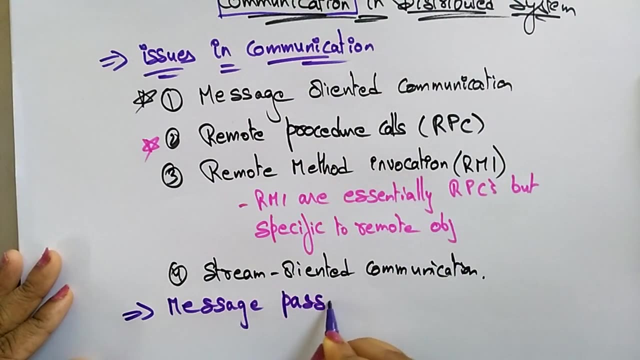 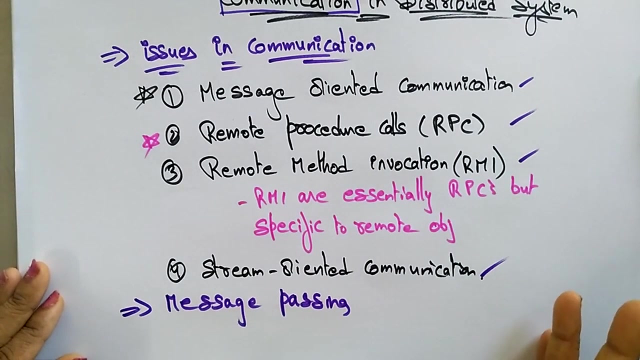 So actually the message. So the message passing is the general basic of communication in distributed systems. So the main general concept here it is a message passing, Message passing. So whatever the type of communication you are taking, So in each and everything the basic concept is a message passing. 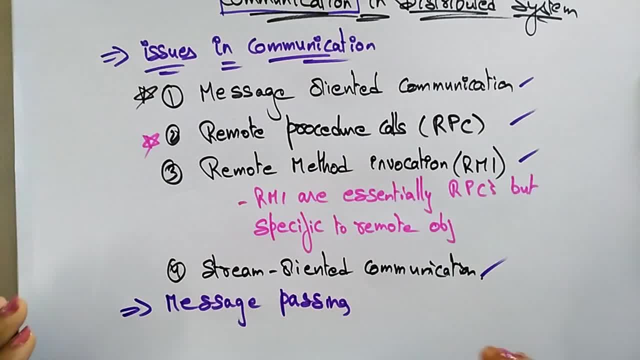 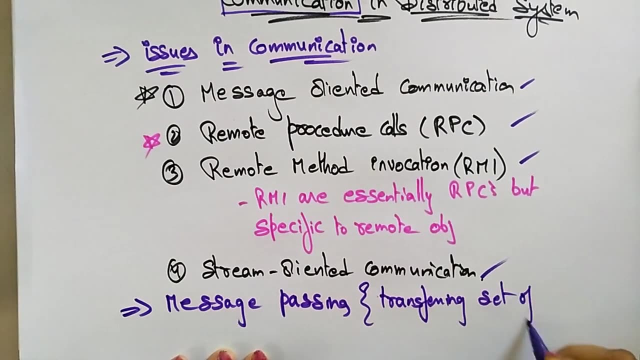 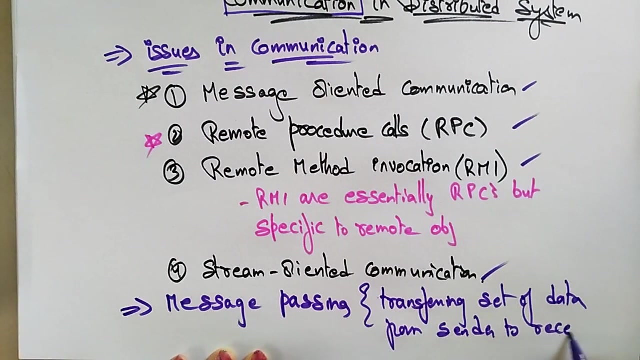 So the message passing is a general basis of the communication in distributed system. That means transmission Transferring, of transferring a set of data from sender to the receiver. Message passing is nothing but transferring set of data from sender to receiver. So just remember this point. 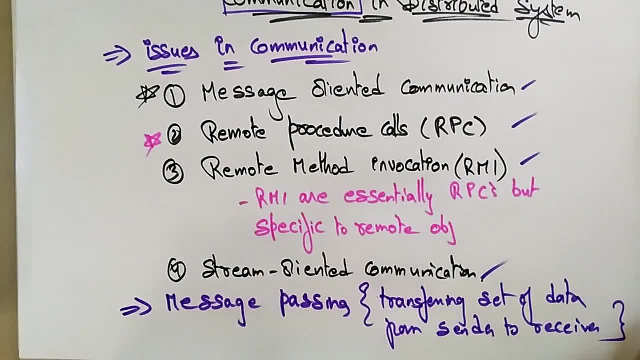 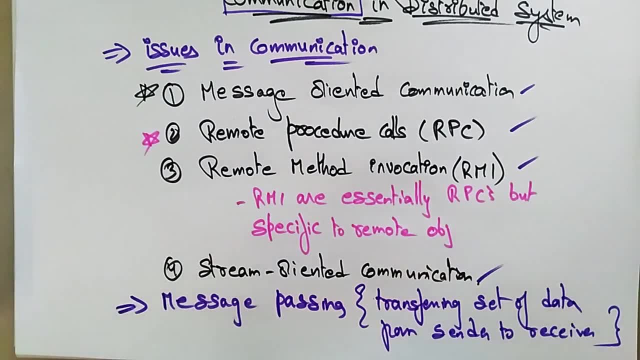 So these are all the different types of communications in distributed system: Message oriented communication, remote processor calls remote method invocation stream oriented communication. So the main basic of communication in distributed system, and whatever it may be, So the main general basic is the message passing. Thank you.